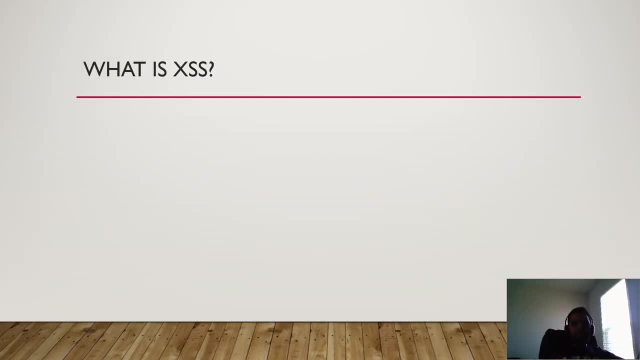 So, in this particular you know video, let's start with the what is cross-site scripting? So, as a rule, XSS occurs when a browser renders untrusted content in a trusted environment. So if the content, is you know, contains any dynamic language such as HTML, JS or any other scripting language, then it would execute inside your you know response or the HTML response, and that's where the XSS occurs. 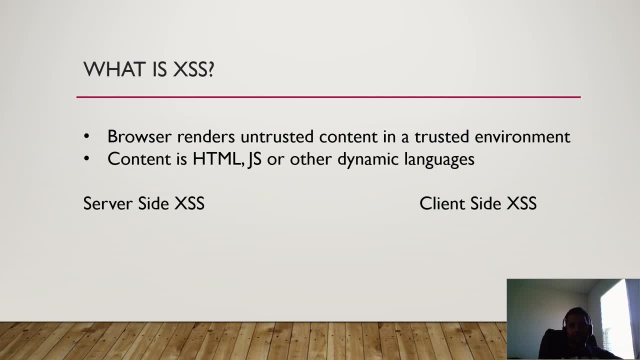 So, like you know, let's talk about the different type of XSS first and then I'll give you some. you know, probably we will go through some sample code on how does the XSS really work. So there are two types of XSS. One is server-side, the second one is the client-side. Server-side again broke it down into two different categories, So one is the reflected, the second one is persistent or stored XSS. 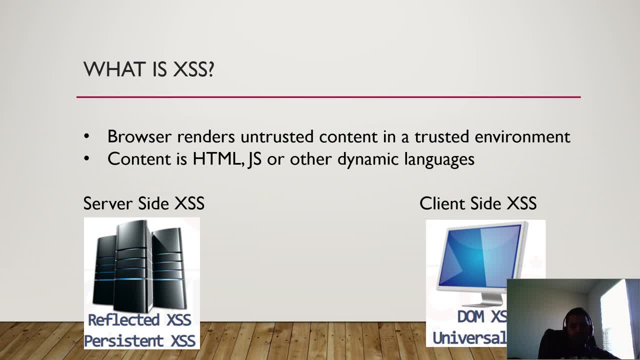 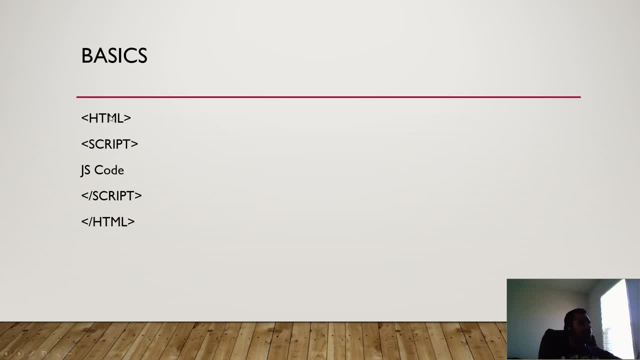 So one is the DOM cross-site scripting, and the second one is universal cross-site scripting. So you have, like you know, href tag or you could pretty much, like you know, write anything. Now within those tags. you, for example, let's say, you know we talk about the JavaScript, like cross-site scripting using JavaScript payload. So within the HTML you have a script tag. 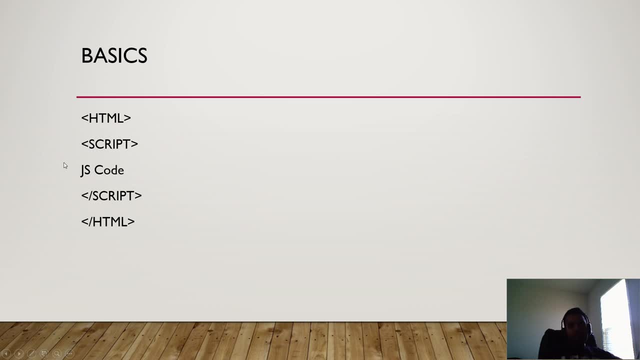 Now in the script tag you are writing your normal JS code on whatever function. So if you are doing a math function, like you know- 3 plus 4 or whatever you have to do- So you can assign values to the variables and you can. 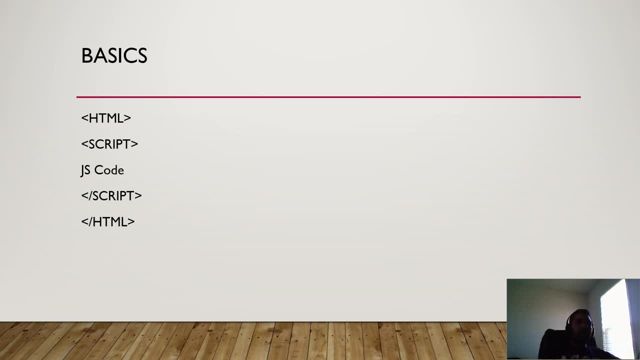 do, like you know, all sort of different operations. Now, in that particular function, if you are accepting a user input and you are not validating it, of course, like you know, that's why cross-site scripting happens, Like you do not filter the user input. So let's say you are accepting, you know, any value from the user, for example, any string. Now, user provides a string, Now being an attacker instead of providing a string. 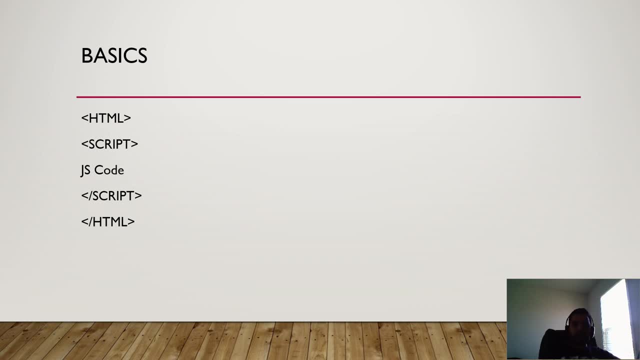 I would provide a JS payload, which could be, you know, alert123 or alert you are hacked, or anything. So that's that one now will be part of this you know HTML page and within the JavaScript tag: Now, when that page will be rendered on your browser, on the user's browser, it's going to execute and it's going to do the whatever attacker has provided as an input. 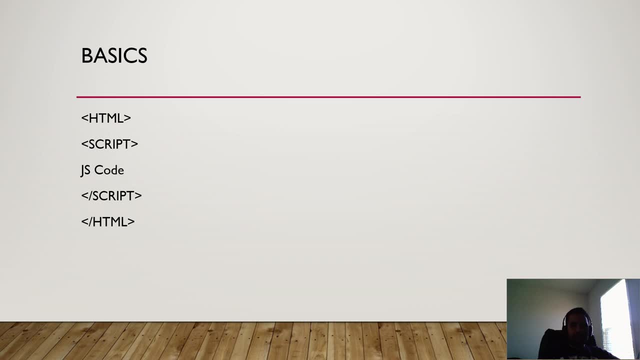 Now, using cross-site scripting, you can do several things. So, like you know, if attacker wrote a script where it could steal the user's cookie value and you set it back to the server that the attacker is managing it, So like you know, it's going to send all the cookie information whenever a user is being tricked or exploited. 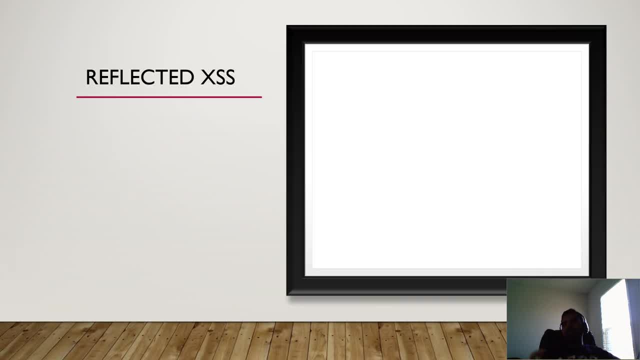 Now let's talk about, like you know, different type of access and what could like, how each one could go wrong. So with the cross-site scripting, uh, reflected, uh, here is the workflow. So how it works is: first, attacker would create a malicious link. 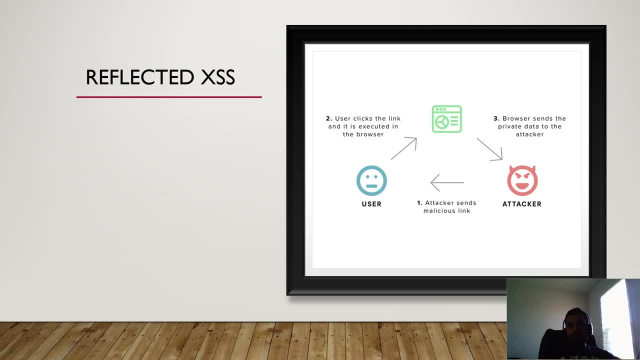 So for example, let's say stp, xyzcom, uh question mark, there is a search parameter, So search is equal to uh script, alert 123 script. So they'll send it to user. user clicks on it. it will, of course it will. the request will go to the xyzcom. 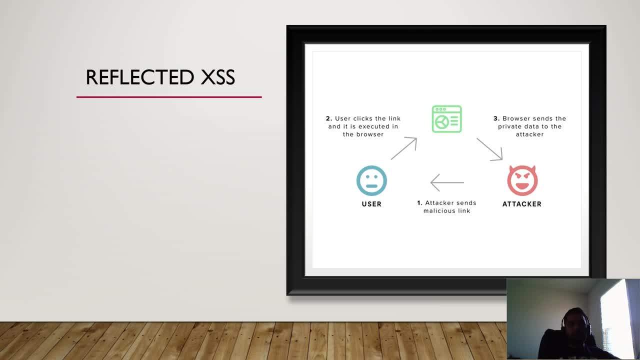 There are no weldings, There is no validation on the server side. So, uh, like you know, I the input, so, whatever the input was to the search parameter, alert 123 will be like, executed on the user's browser. 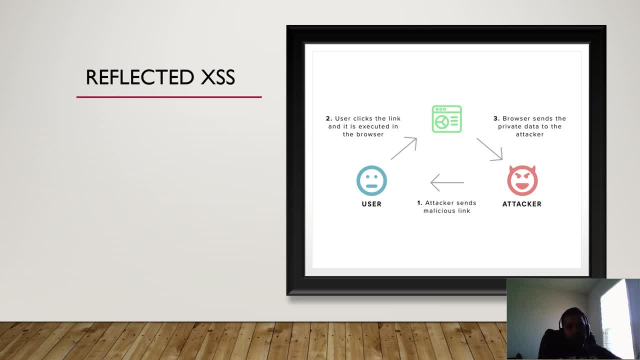 Now, as I saw, like you know, as I told you before, so attacker could get uh cookie information, could steal cookie information. So in that case, uh, it's going to be executed and the website will send all the information. like you know, browser sends all the private data to the attacker. 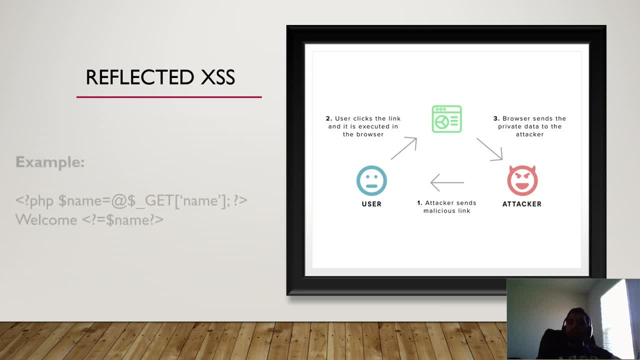 Uh. but to make it work, like you know, uh uh, reflected cross-site scripting attacker has to be smart, because if you send someone uh where, where you know, in the search parameter, it can clearly see that there is some sort of you know, fishy payload, like alert and script and all those things, then user won't click on it. 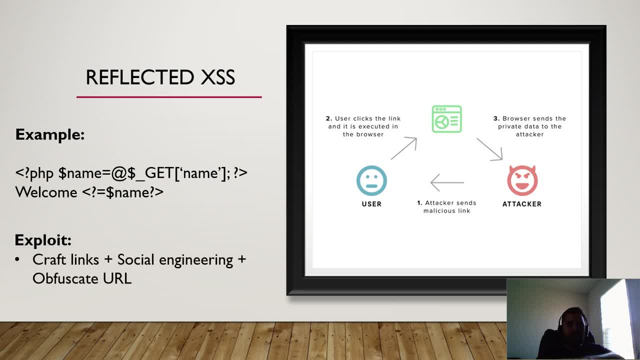 So you would have to trick the user, So you would have to craft the links, Then you have to, like you know, social engineer, Then you have to, like you know, user and then you will also have to obfuscate the URL because, like you know, if it's a simple text, plain text URL, anyone can see and understand. this is fishy and they'll not click on it. 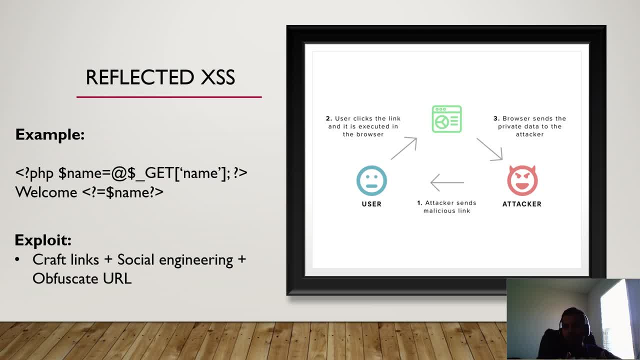 So you have to do all of these things and then trick the user, and that's when the reflected cross-site scripting happens Again. this is you know one time. So, for example, if you have a hundred, if you want to exploit a hundred users, you would have to send the link to the hundred users. 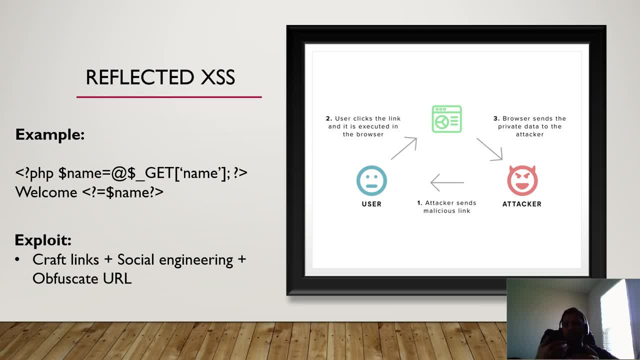 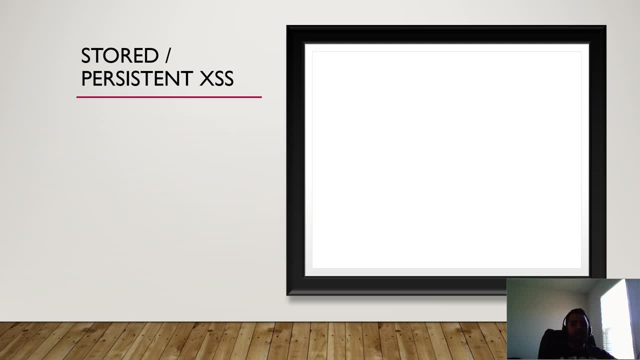 They'll have to click on it. So when they click on it, it's going to exploit. Now let's talk about the stored XSS, and this is my favorite- any attacker's favorite- cross-site scripting. So in this one it's a simple scenario. 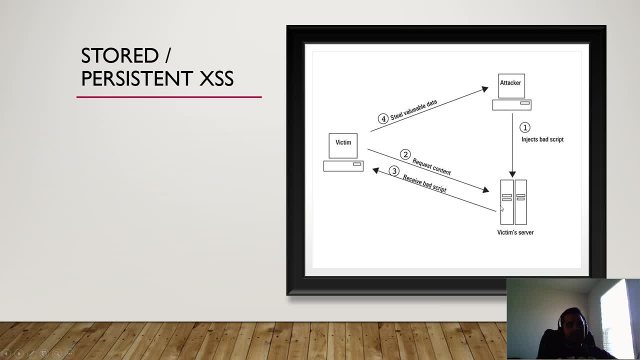 So let's say, you know, here's the attacker and here's the server. So, like you know, XYZ server, this is the server. And let's assume this application is, you know, HR records. So like it, like you know, it creates a user profile and stores user profile in the database or file system. 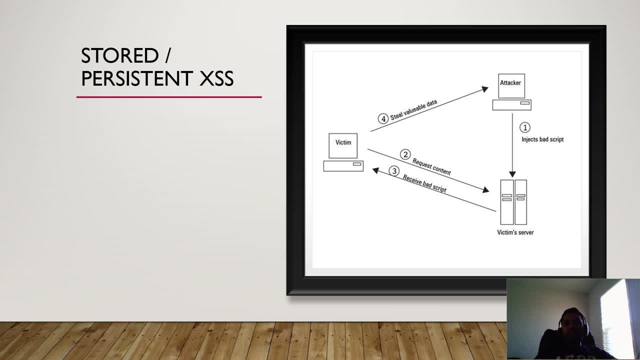 Now what attacker can do is it could inject the JavaScript. So in our example it's a script alert one, two, three or, like you know, script alert document at cookie or script doc. Like you know, you could also redirect user. 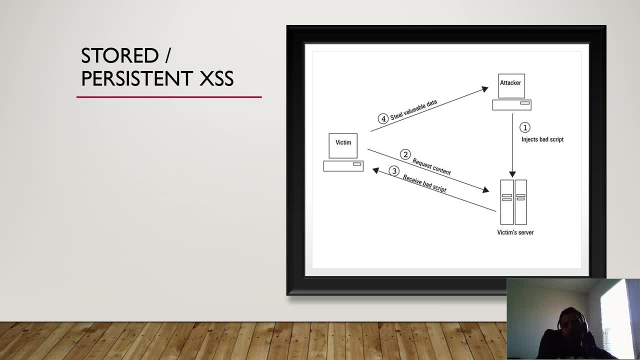 You can also deface the entire application- Pretty much anything you can do. So, attacker being have access to that particular site, it's going to inject the script into the victim server. So now that payload is now saved in the database, 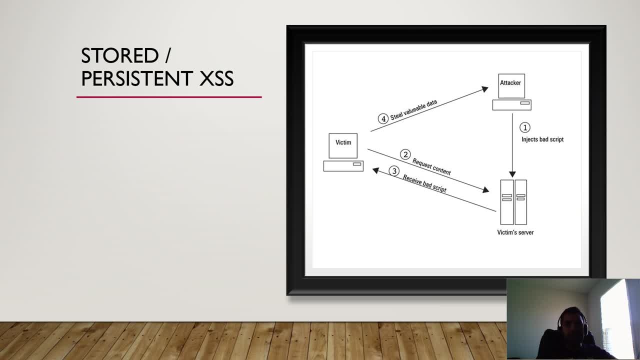 So, like you know, you are not so in the reflected we were sending this payload to the user. Here we are storing that payload into the victim server in the database system. Now imagine whoever have access to the XYZcom or whoever accesses this page, is going to get. 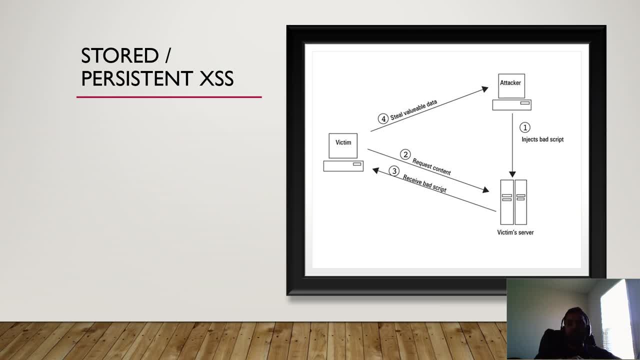 you know exploited because whenever you know user is going to go to the view user profile page or any page where it would fetch the record from the database. along with the records, it's going to also fetch the script which attacker has injected here at the first place. 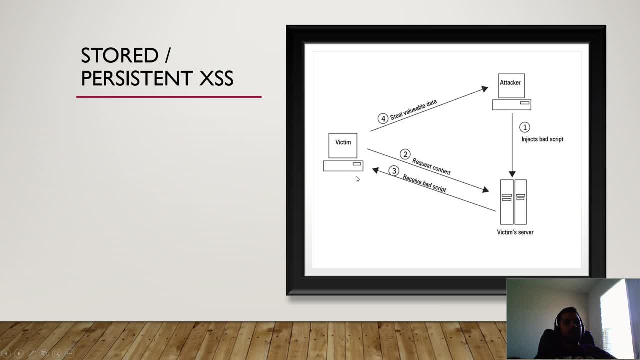 So now, like you know, server will send the bad script to the victim and victim will get exploited. Now, the reason I said, like you know, it's my favorite, because one time you inject the script into the victim server, you know it's going to get exploited. 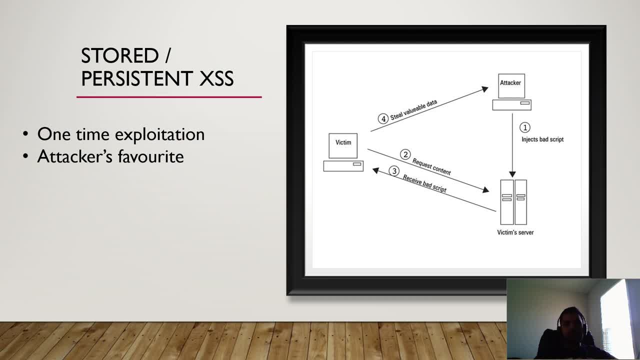 So now, like you know, server will send the bad script to the victim and victim will get exploited. You know, you inject the script and then you don't have to worry about the social engineering. You don't have to worry about, like you know, crafting the link sending to the user. 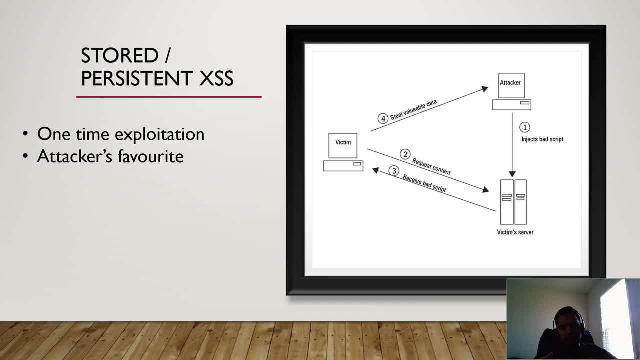 If there are, like you know, thousand people accessing that server or that application, they all will be affected. And this is, like you know, simple, like the simple example of this could be a blogging application, So where you have the blog, after the blog is completed, you are allowed to write the comments. 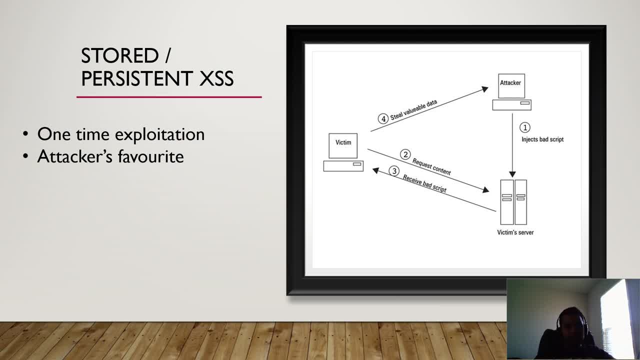 And if the comment box is not protected, I can write my script and I can save it to the server and every time, whoever reads the blog, they're gonna got exploited. so that's how simple it is. now wasp has a good example that we just 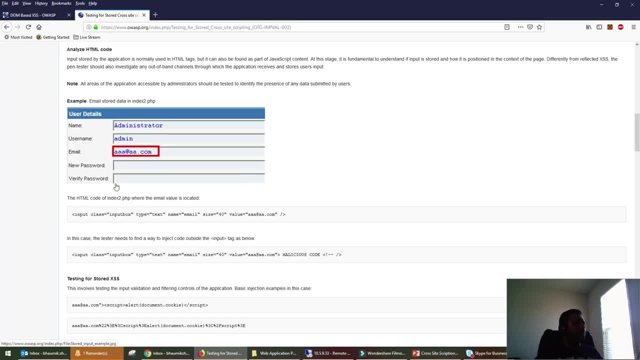 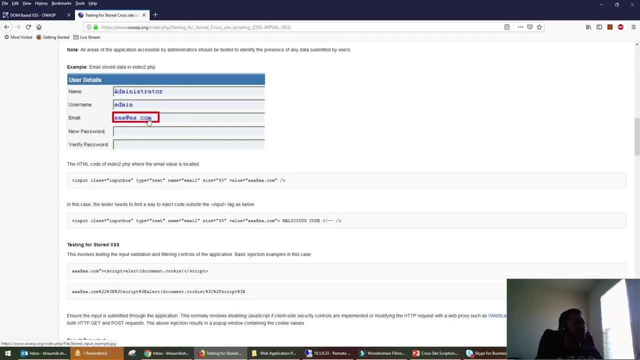 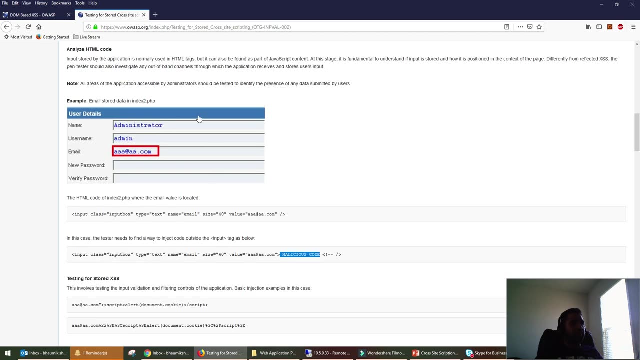 talked about. so if you want to take a look, so here it is, so if you see here. so this is the page of the application and instead of email, like you know, valid email. let's say, we enter some malicious code, so, like you know, it's got stored to the backend system and every time someone open up, 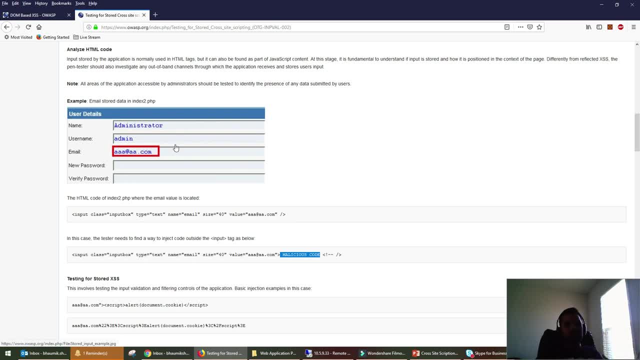 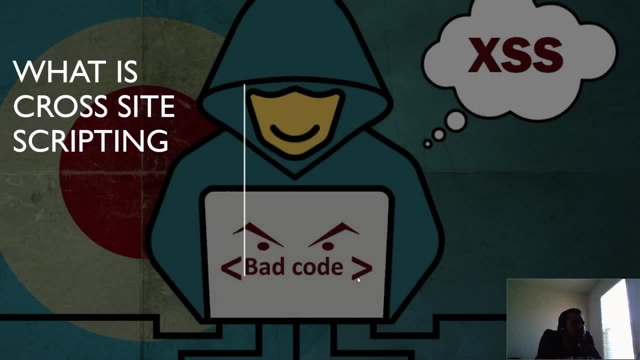 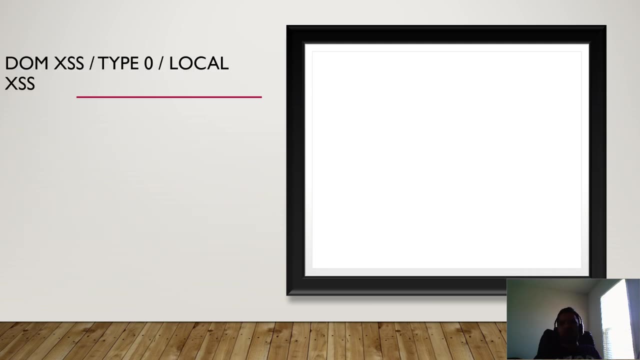 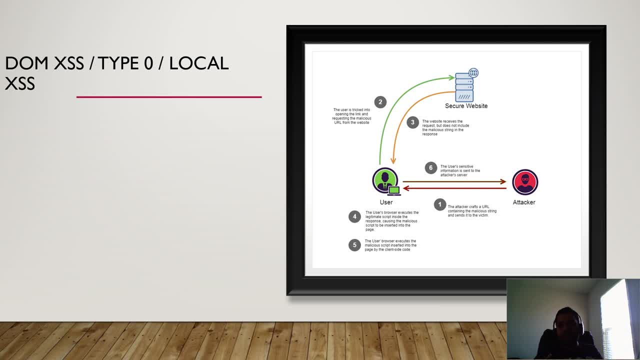 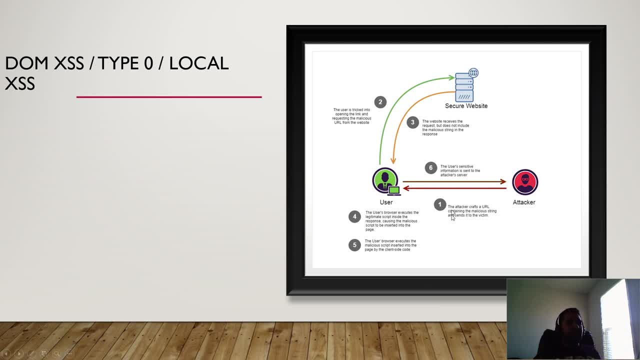 So now what happens here is the attacker is gonna grab the URL containing the malicious string and send it to the victim. Now victim is going to click on it. So this is so far. This is similar to reflected cross-site scripting, So victim, or the user, is going to click on it. 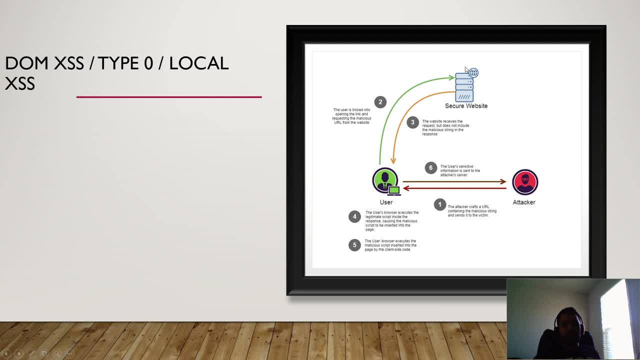 It's going to this: like you know, server, like application server or the website Website, receive the request, but does not include malicious string in the response. Because, you know again, this is not a server-side for novelty, This is a client-side code, where you have something written on the client-side page, where you are using JavaScript or something. 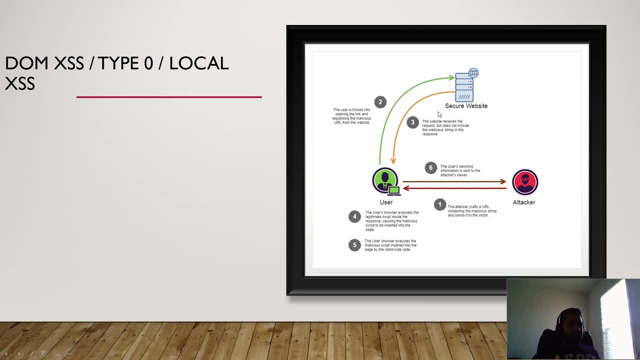 And that's being exploited. So the website you know sends back, sends the response back to the user, or I would say users browser. now, the user browser execute the script inside the response, Causing the malicious script to be inserted into the page. So, and like you know, again so malicious script, whatever it is, it's gonna get executed. 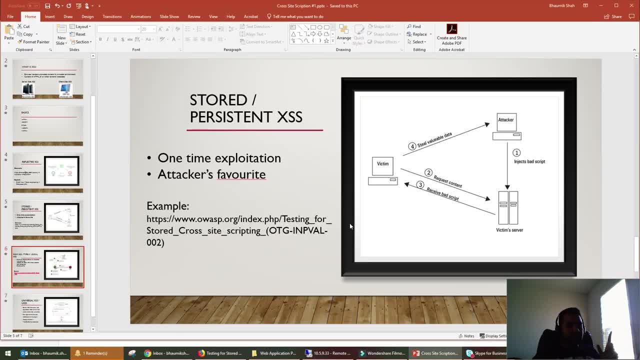 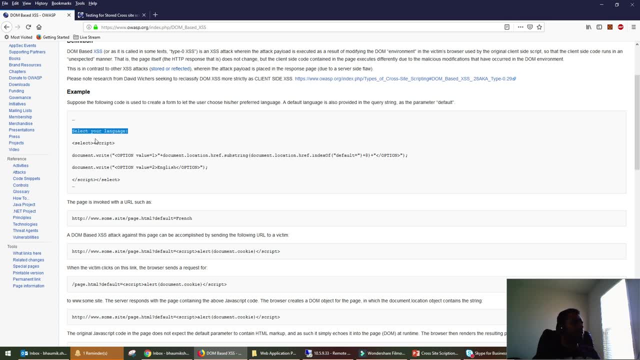 So here that the thing is alright. so let's first take a look at the example here. So I'll go back to the OWASP site. Well, we have the example. So, for example, in this website you could select the language. so it allows you to select the language. and there's a little you know. 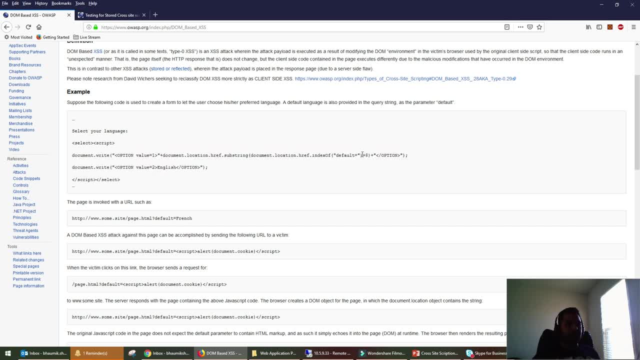 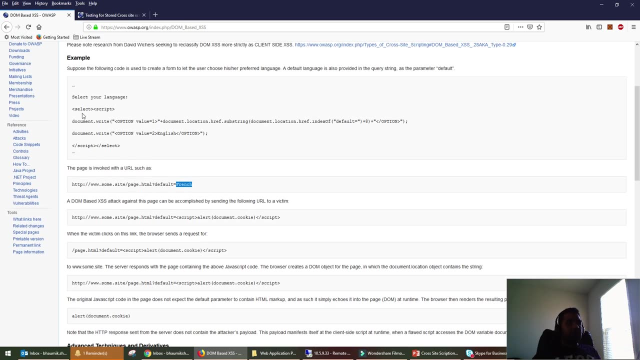 JS code here. So in this JS code You could select the language. So you know the default parameter. here You could select language: probably French, or you know English or whatever. it is Now the. the key part here in the DOM exercise is: this is a client-side code. 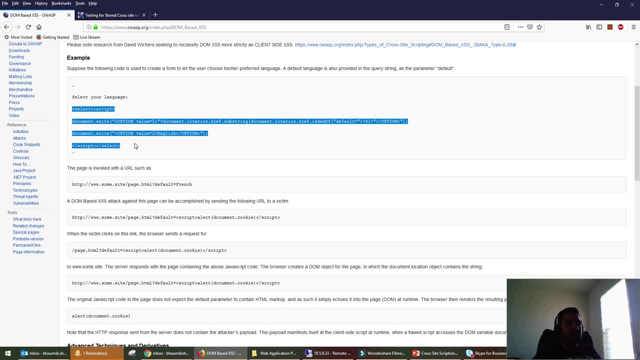 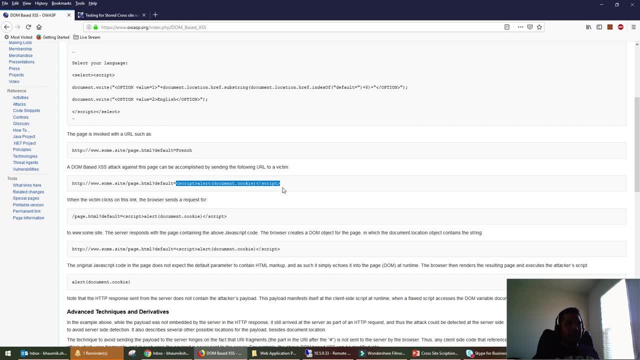 Like: this is not somewhere stored on the server side, So that's a difference. So now, in this value like instead of French, what if the attacker writes this one? it will obviously get executed, because you know there is no protection here. and when browser says this value, it's gonna fetch the cookie from the DOM and give it back to the. 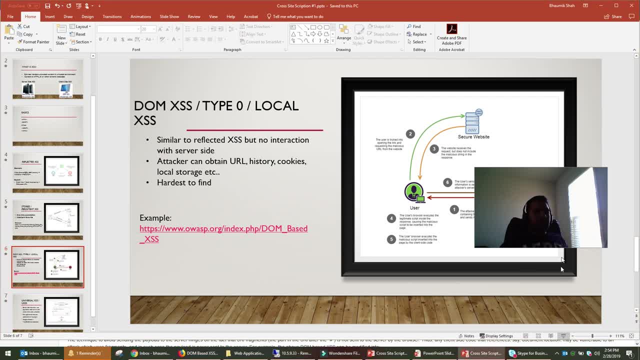 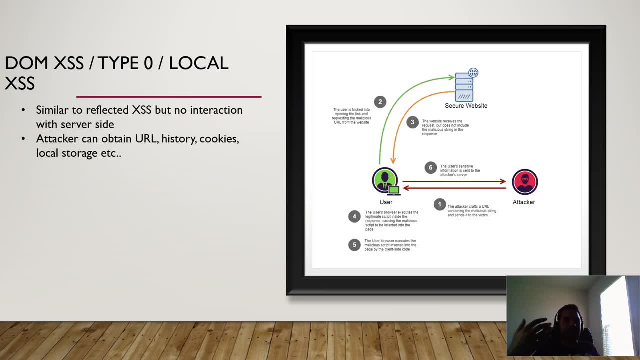 Attacker. so that's how it works. now Let's see you know what attacker can gain, like you know, after exploiting all these things. So attacker could obtain URLs. attacker could obtain History, cookie information, local storage. So I've also seen, you know, Many software developer attend to save a lot of sensitive information in the browser local storage, which is not a good practice. 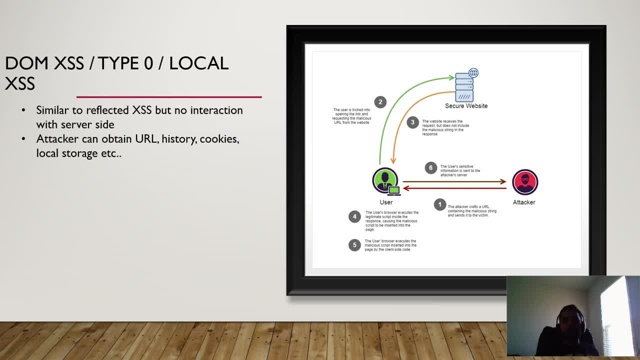 It should be avoided because if you happen to have a DOM access, as somebody could steal all this information- The only thing with the DOM access is it's very hard to find, like you know. Of course, you can take help of the automated tools, which would make your task. 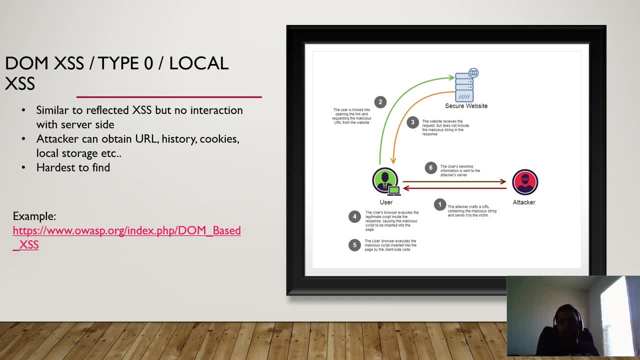 A little easier, but still it's. it's very difficult to find DOM based access. in my experience I Have you know out of ten applications I would find six or seven times reflected or stored. then the DOM accesses. But of course, like you know, feel free to visit this link on the OWASP site. 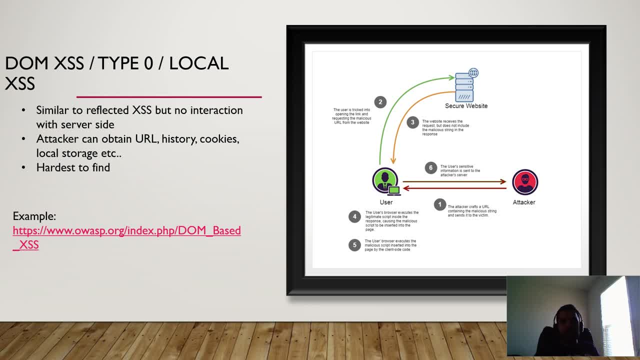 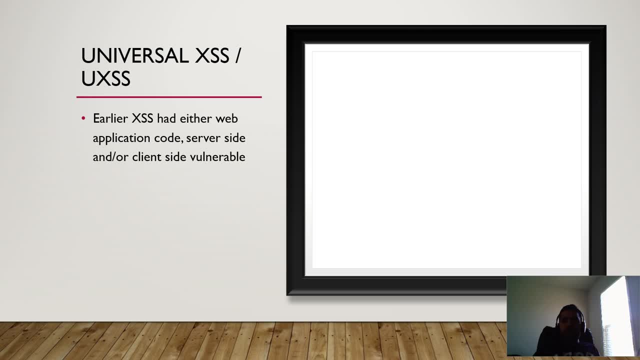 They have a good example and explanation as well, in case you have any further questions. and let's talk about the last one, Which is universal XSS. So earlier, whatever XSS we talked about- reflected DOM or stored XSS- They had to do something with the application code, server-side code or client-side code. 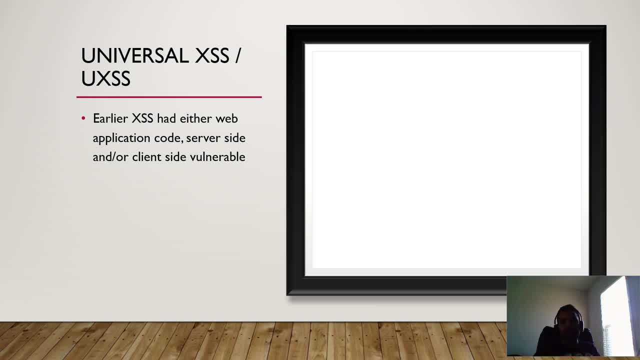 You know. but this one it's little different, because here you are dealing with the plugins or extension. So nowadays we all use browser and we all use plugins and add-ons, you know, install in the browser. So this cross-site scripting happens if your plugins or browser extension is not secure. 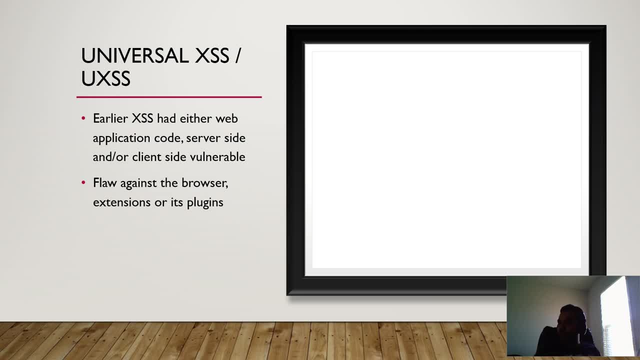 Sometime I always seem like you know application also make use of certain plugins. Sometime I have also seen you know You also get a task of like pen testing plugins, So you have to make sure like plugins can also. if it's a browser plugin, somebody could still exploit it. 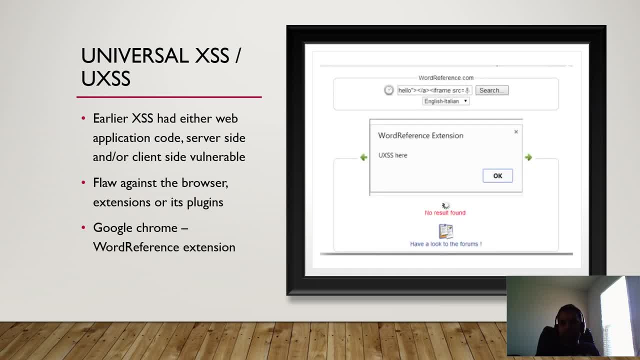 And simple example is, like you know what reference extension Where you can see there is a search box. You can put the payload in there and then you know, someone can easily exploit because there is no protection there. So this is pretty much all I wanted to talk about, like you know.